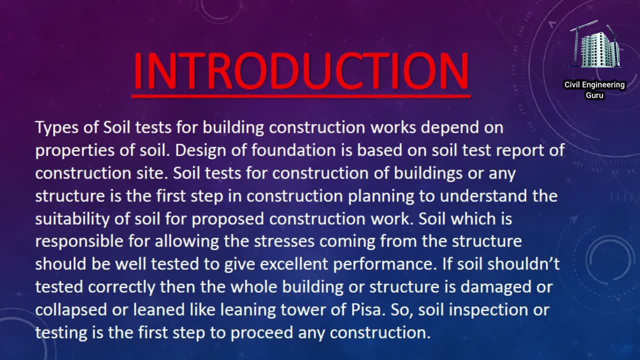 First we talk about introduction. Types of soil tests for building construction works depend on properties of soil. Design of foundation is based on soil test report of construction site. Soil tests for construction of buildings or any structure is the first step in construction planning to understand the suitability of soil for proposed construction work. Soil which is 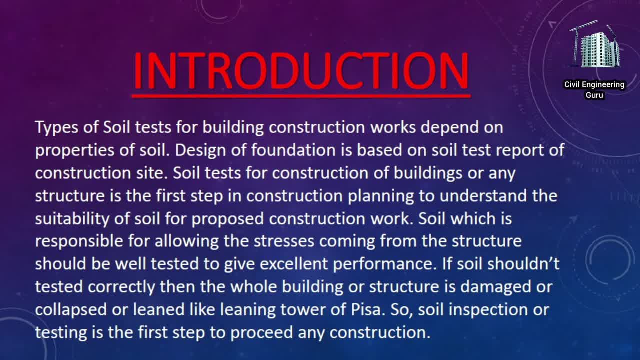 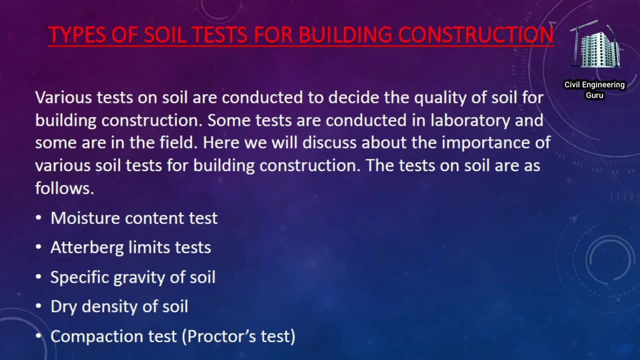 responsible for allowing the stresses coming from the structure should be well tested to give excellent performance. If soil shouldn't tested correctly, then the whole building or structure is damaged or collapsed or leaned like leaning tower of Pisa. So soil inspection or testing is the first step to proceed any construction. Now move toward the topic types of soil tests. 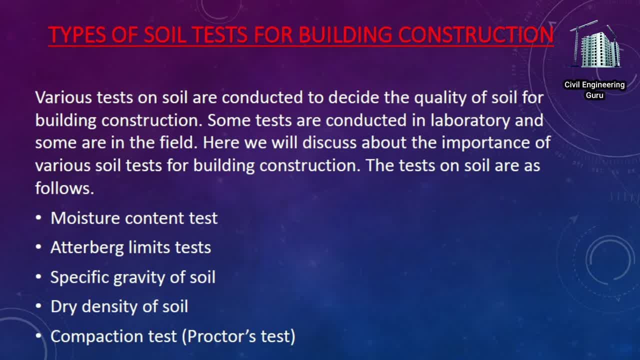 for building construction. Various tests on soil are conducted to decide the quality of soil for building construction. Some tests are conducted in laboratory and some are in the field. Here we will discuss about the importance of various soil tests for building construction. The tests on soil are as follows. 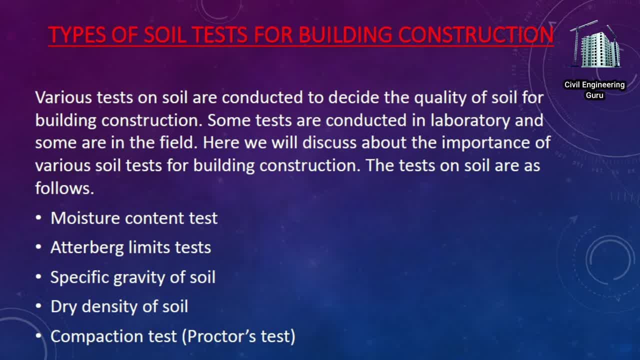 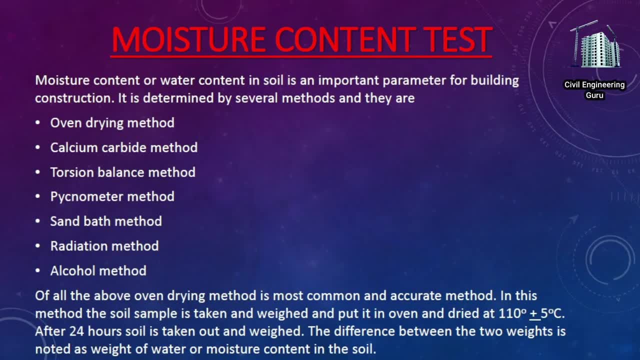 Moisture content test. Adderberg limits tests, Specific gravity of soil, Dry density of soil, Compaction test. Proctors test. Now move toward first type of soil test: moisture content test. Moisture content or water content in soil. 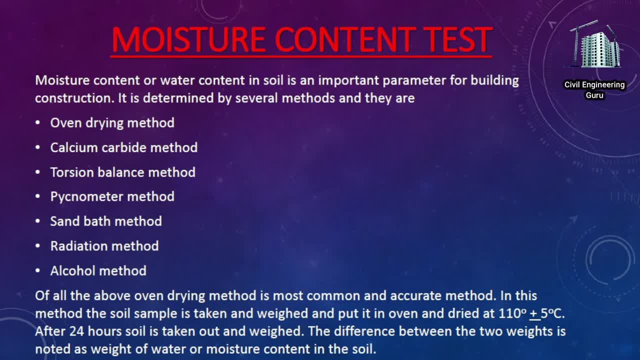 is an important parameter for building construction. It is determined by several methods and they are: Oven drying method, Calcium carbide method, Torsion balance method, Pycnometer method, Sand bath method, Radiation method, Alcohol method. Of all the above, oven drying method is most common and accurate method. In this method, the soil 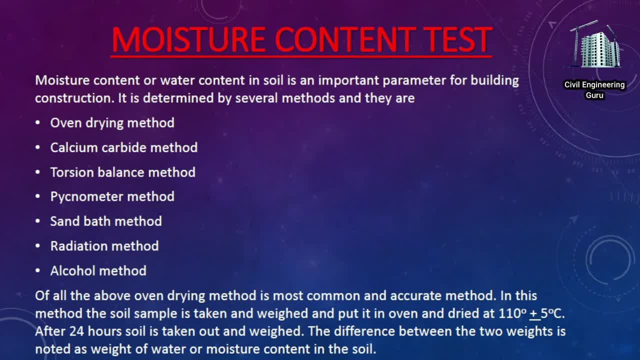 sample is taken and weighed and put it in oven and dried at 110.05 O C. After 24 hours soil is taken out and weighed. The difference between the two weights is noted as weight of water or moisture content in the soil. Now move toward next type Atterberg limits tests. The Atterberg limits are: 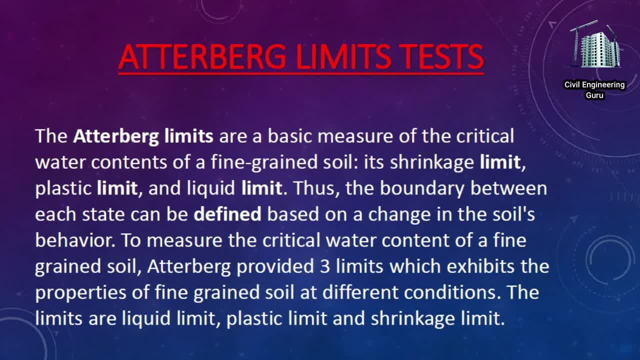 a basic measure of the critical water contents of a fine-grained soil, Its shrinkage limit, plastic limit and liquid limit. Thus the boundary between each state can be defined based on a change in the soil's behavior. To measure the critical water content of a fine-grained soil, Atterberg provided. 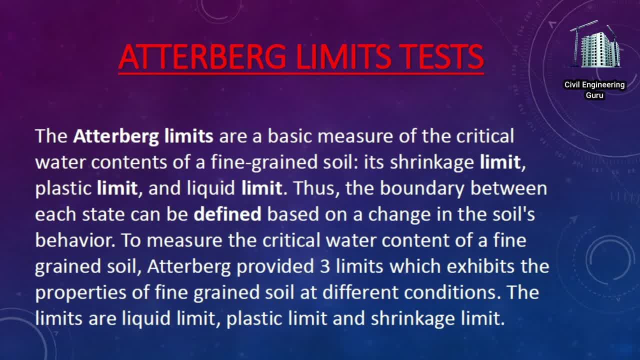 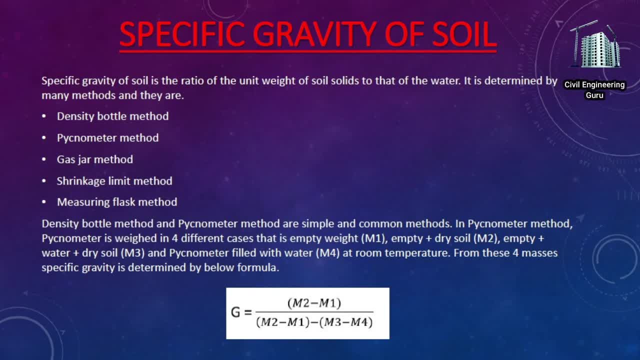 three limits, which exhibits the properties of fine-grained soil at different conditions. The limits are liquid limit, plastic limit and shrinkage limit. Now move toward next type: Specific gravity of soil. Specific gravity of soil is the ratio of the unit weight of soil solids to that of the water.